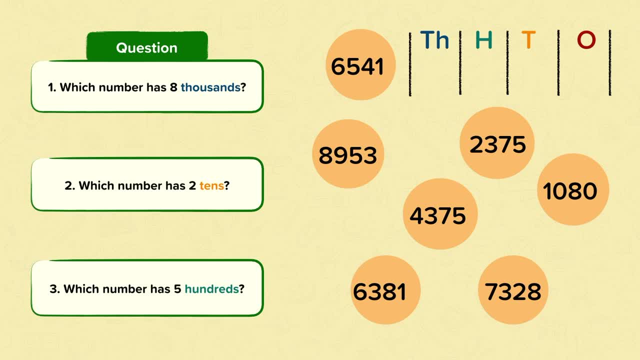 number has five ones. Can you find which number has two tens and which number has five hundreds? Pause the video if you need to. Well done if you knew that 8,953 has eight thousands, 7,328 has two tens and 6,541 has five hundreds. 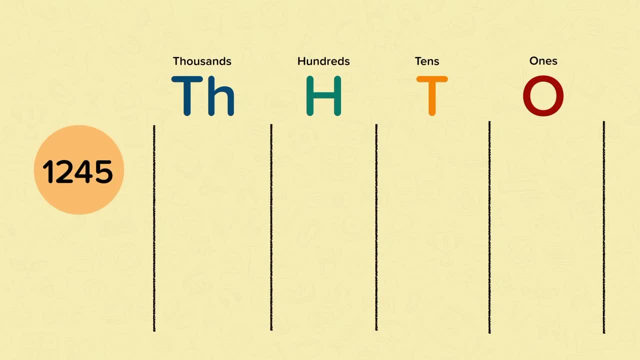 Let's have a look at this number now: 1,245.. So it's got 1,000, two hundreds, four tens and five ones. Now let's use pictures to represent this number. So it's got 1,000, two hundreds. 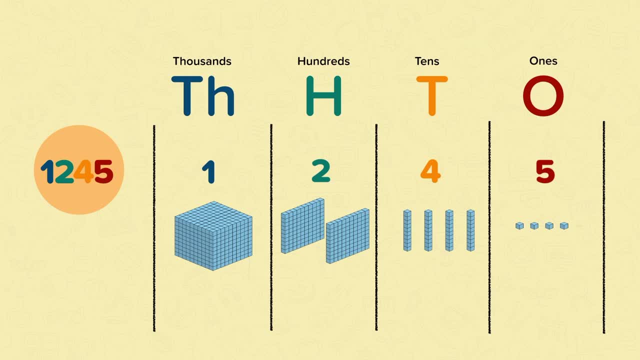 four tens and five ones. Now let's have a look at the value, The value of each digit in this number. So the value of the one in the thousands place is 1,000.. The value of the two in the hundreds place is 200.. The value of the four in the tens. 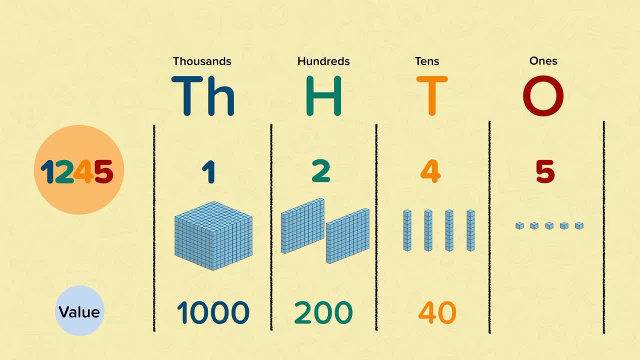 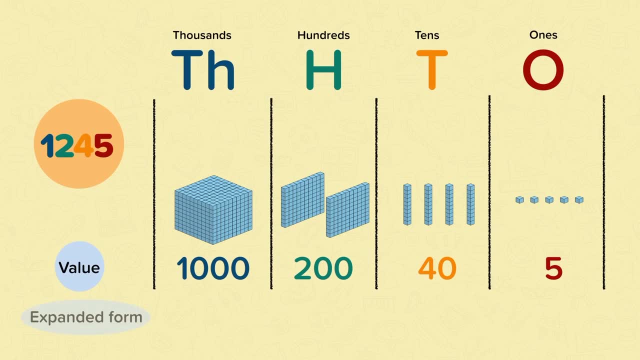 place is 40. And the value of the five in the ones place is just five. Pause the video if you need to. The expanded form is used to show the value of each digit in a number. So 1,245 written in the expanded form would look like this: 1,000, add 200, add 40,, add five, Or it could be written: 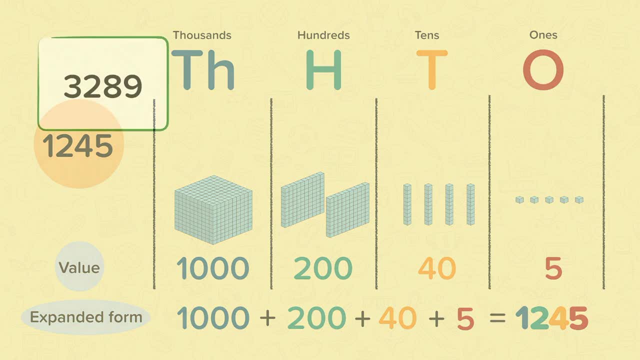 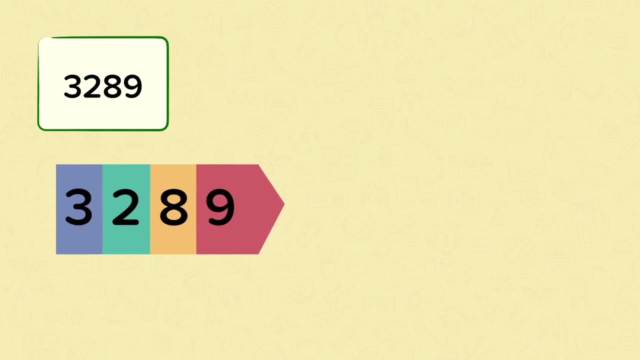 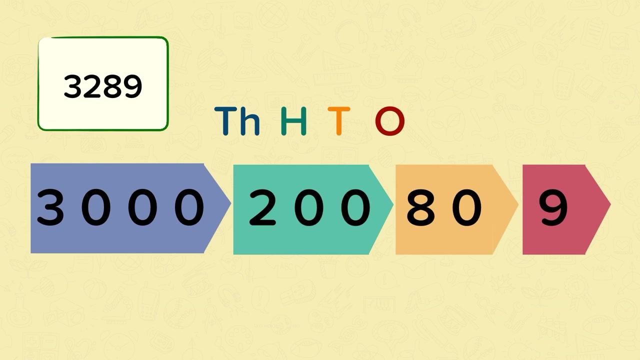 the other way around to look like this. Now let's have a look at this number: 3,289.. This time we're going to use place value cards to help us to understand the value of each digit in the number. If we pull this number apart, you can see that this number is made up of 3,200,, 80 and 9..